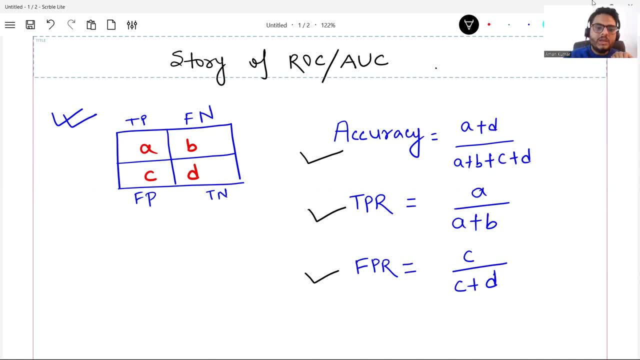 then you might be observing that these numbers are fixed. Okay, So in your confusion matrix, every time you plot a confusion matrix right, you will see these numbers are fixed. For example, 1203, let's say five, and this is 115.. Have you ever given a thought that in a probabilistic 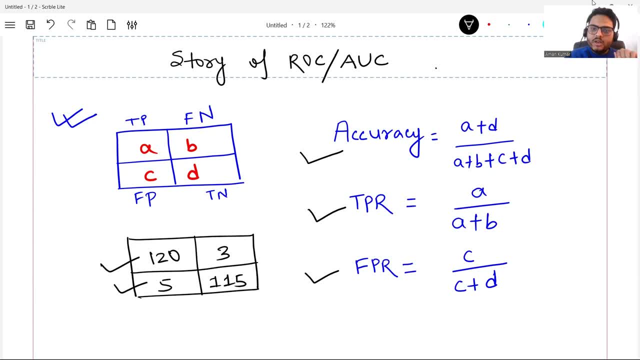 model how these numbers are getting fixed. Now you might be understanding from the hint I'm giving to you that, based on some probability threshold, these numbers are fixed Right. So how these numbers come, how do you know which is true, positive, which is false? positive? 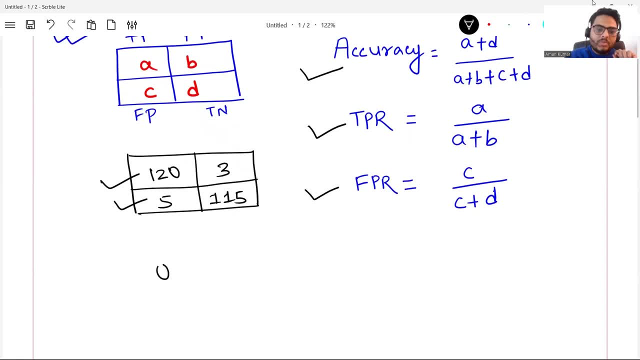 you know, by setting up a threshold right, The threshold by default is 0.5.. So any observation which is above 0.5 probability, we call that as one class below 0.5, we call that as zero class. 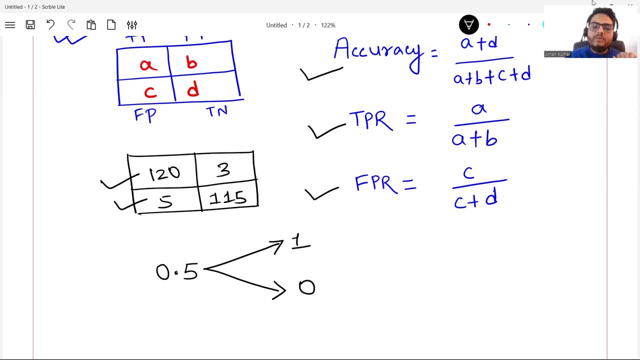 Okay, This is very simple to understand concept. Now, if I make this 0.5 as 0.4, then all your numbers will change. right, All these numbers will change. Okay, Try to digest these guys. Then I will go to the main concept. Okay. 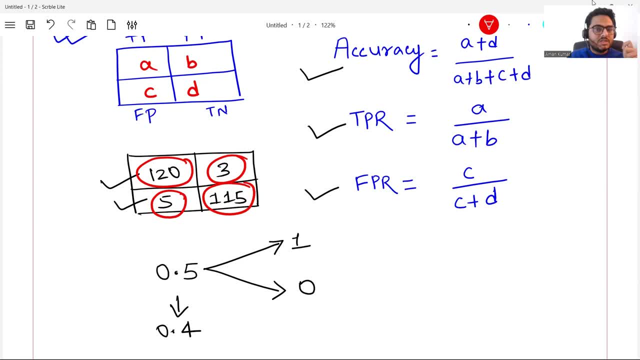 If the threshold is changed, then your confusion matrix changes. If your confusion matrix changes, then your accuracy changes, your TPR changes and your FPR changes, right. And somebody asks you: Hey, give me one metric that can tell me how good your model is, If I make any threshold. 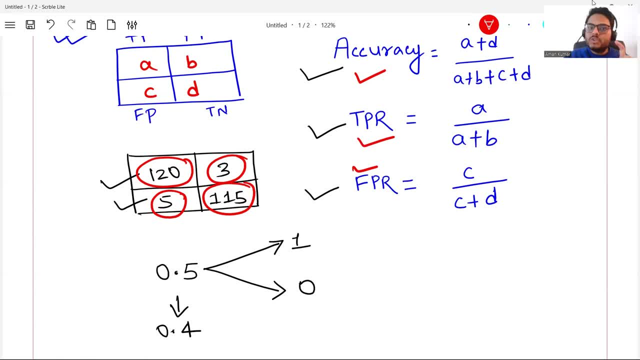 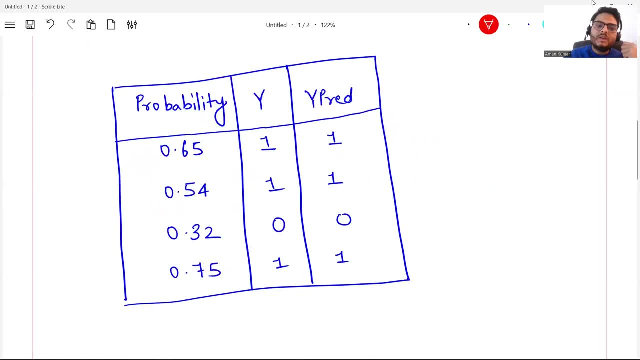 for example, your metrics would not be depending on the threshold. You give me one metric that is independent of threshold. Okay, Let's try to understand with a simple example here. Suppose these are the probabilities, Okay, And this is your Y actual and this is your Y predicted. 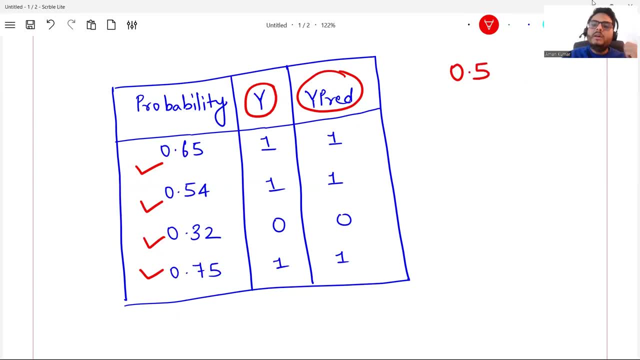 Suppose yours. your threshold is 0.5.. Okay, If your probability is above 0.5, you call that one class or you call that zero class. Now, if I ask you from 0.5 probability, what is the accuracy of this model? So everything looks fine. One is predicted as one. 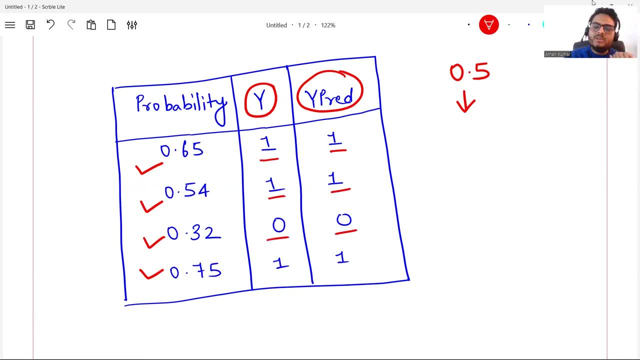 Below 0.5, zero is predicted as zero. Above, one is predicted as one. At the moment, I tell you, Hey, at probability 0.55, I want to make my threshold. So I want to change my threshold from 0.5 to 0.55.. At the moment I do this, this one will be predicted as zero and this prediction. 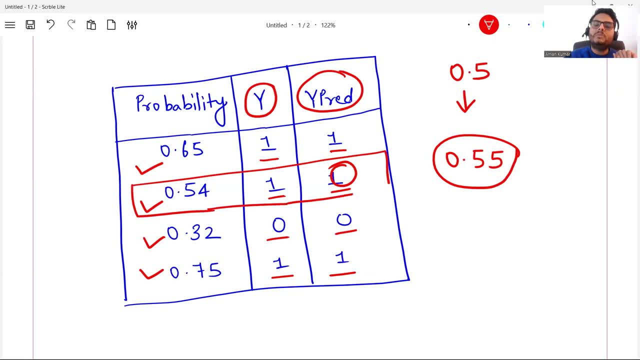 will go wrong and your accuracy will come down and all your TPR, FPR will get impacted. To find a solution for this, we need a number that can tell me how good is my model through the range of threshold. Okay, It is threshold, independent measure of X. you know, assessing your model. 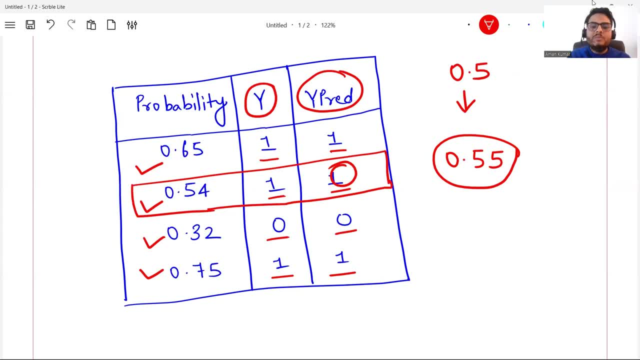 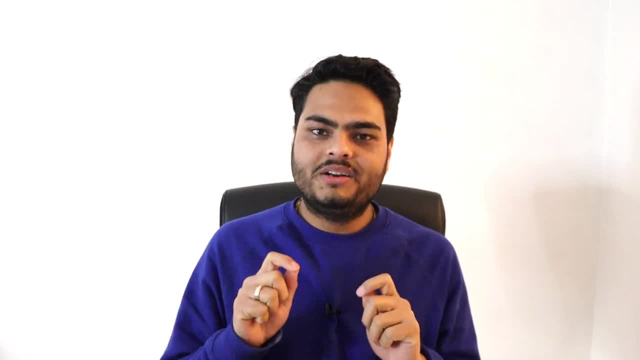 you can say or, or finding how good is your model? Let me quickly show you in Python What I mean by that. Okay, Sorry for interruption, guys, but just one request: If you have ever liked any video at unfold data science, after you complete this video. please share this channel in the comment section below. If you like this video, please share this channel in the comment section below. If you like this video, please share this channel in the comment section below. If you have ever liked any video, please share this channel in the comment section below. 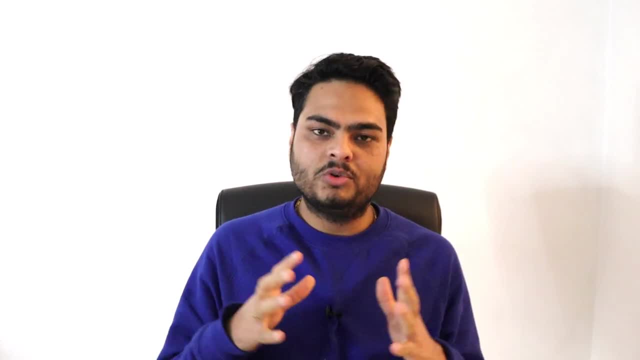 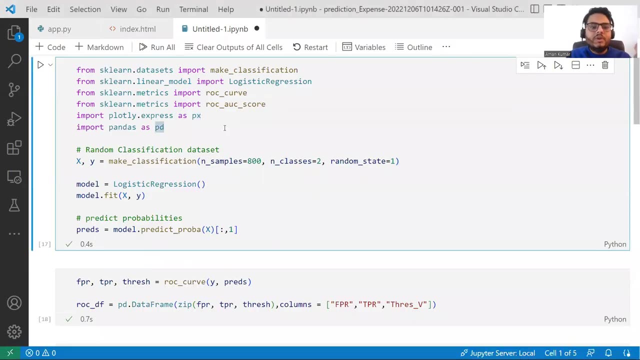 One group beat one WhatsApp group, or beat one telegram group, or beat one Facebook group or LinkedIn page. please do that, guys. So here guys, if you can see, I am taking a simple SQL and dataset, some logistic, regression, model, metric and ROC IOC score. I'm taking something to plot. that plot is interesting plot You will. 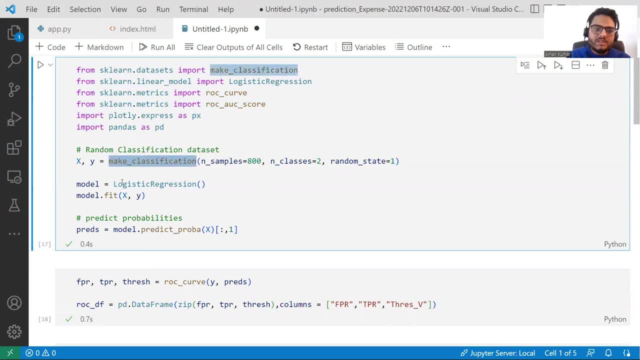 see towards the end. Okay, And I'm doing a classification, data, generating logistic regression and fitting. Okay, Let me fit this model here. Model is fit And if you see, here I'm saying FPR, TPR and threshold is equal to ROC curve wipe rate. So 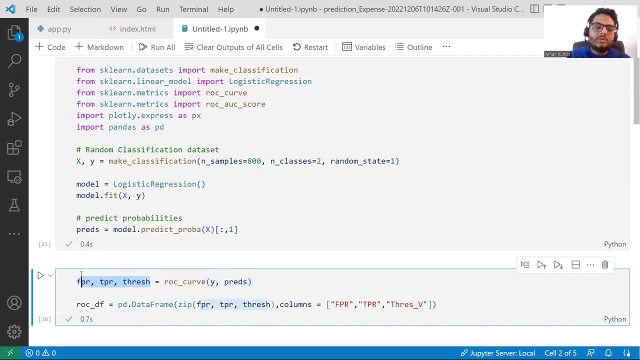 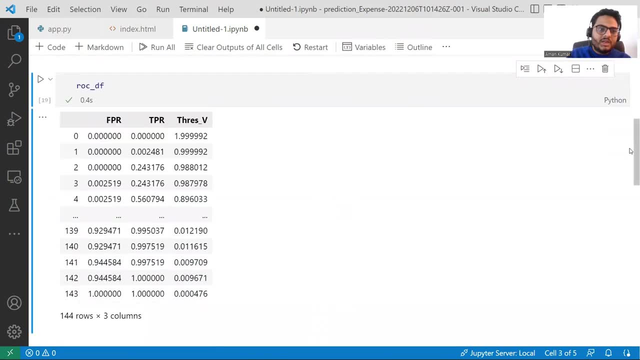 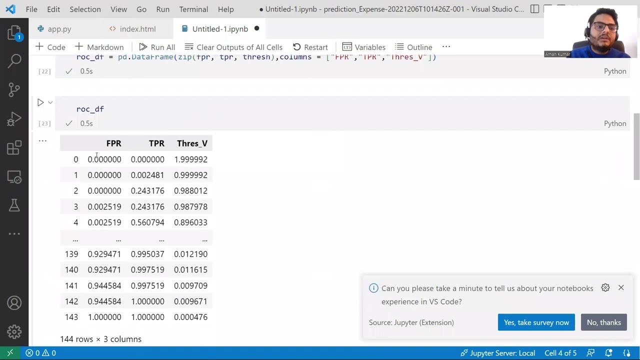 all these three things a skill, and we'll give you, okay, Threshold also, FPR, TPR also. Now I'm creating a ROC, DF, ROC data frame. If you see here, this is my ROC data frame that you are seeing here. Okay, This is my ROC data frame. So what this data frame tells you is at this FPR. 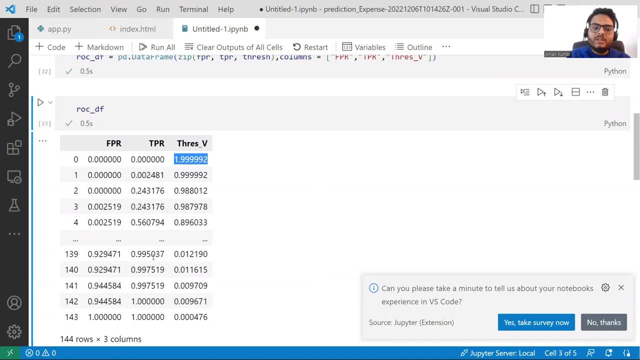 and this TPR. this is the threshold at this FPR and this TPR. this is the threshold. So at the moment you change your threshold, your FPR and TPR starts changing. So all those combinations I have put in this data frame you can say: and in the bottom: 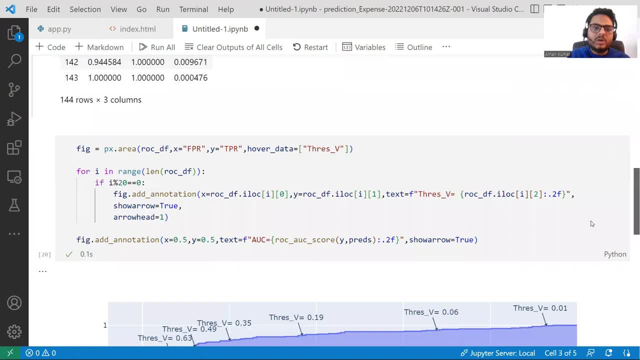 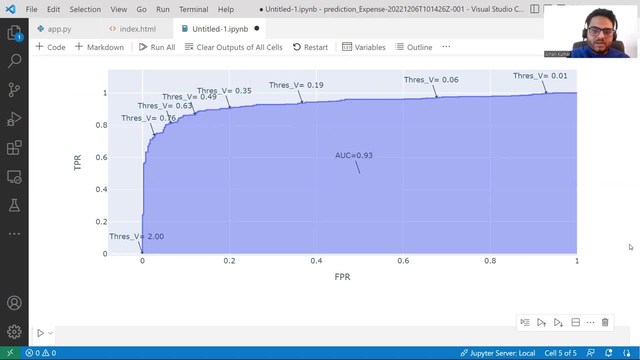 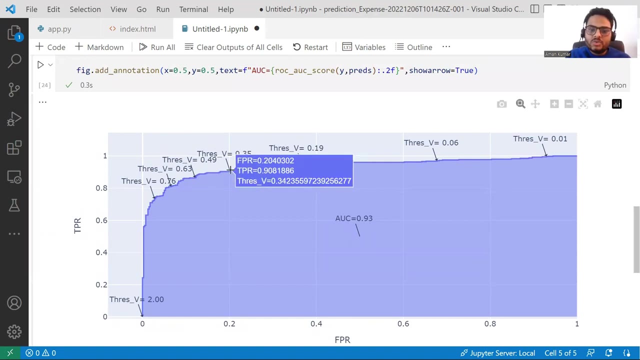 I am plotting that. Okay, Don't worry much about what I have written for the plotting code, Just try to understand how this is getting plotted. Okay, Now see these guys very carefully. This is an interesting chart here. Okay, Threshold FPR and TPR is this at threshold 0.34.. Your FPR is: